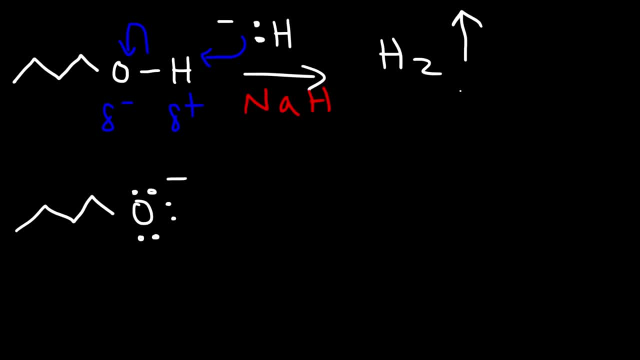 Now hydrogen gas will leave the solution. It's just going to go up there, And then, in the second step, we can react this with an alkyl halide like ethyl bromide, And so this step is an SN2 reaction, which means we need to use methyl and primary halides. 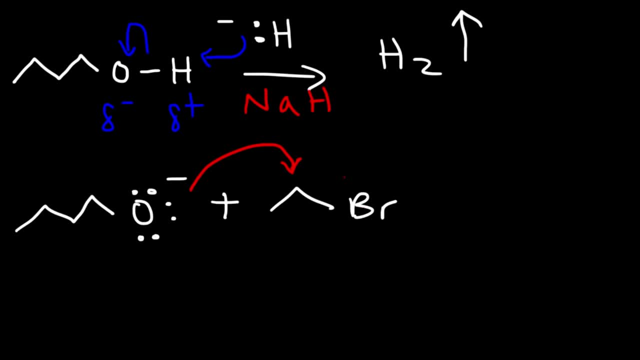 Secondary halides could favor an E2 reaction. So you don't want to use a secondary alkyl halide And this will give us an ether, And so that's the basic idea behind the Williamson ether synthesis reaction. Now let's work on another example. 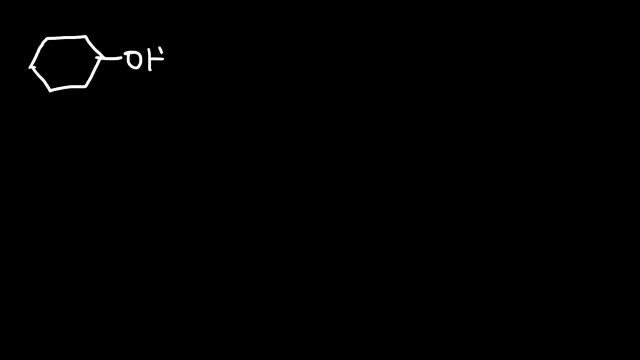 Go ahead and try this problem. Let's say, if we have phenol and we're going to react it with sodium hydroxide in the first step, and in the second step we're going to react it with methyl bromide, Go ahead and predict the. 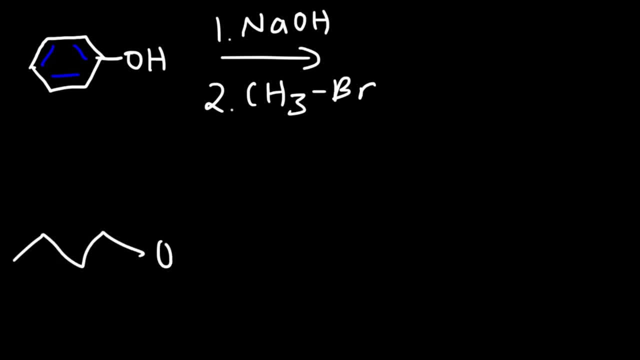 major product. Now for the last example. we use 1-butanol, and the pKa of most alcohols is around 16 to 18, and so for this you need to use a strong base like sodium hydride or sodium amide, Sodium hydroxide. if you use it, the reaction will be in equilibrium. 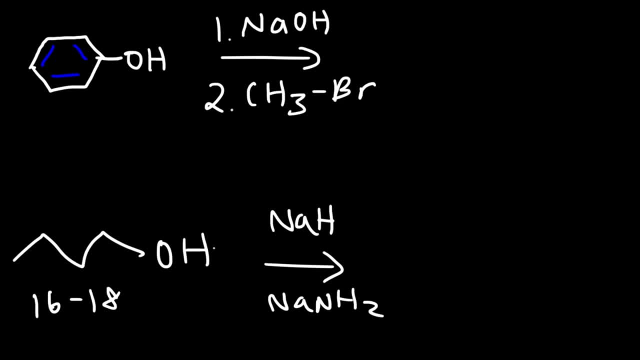 It can take off the hydrogen, but not in good yield. The pKa for phenol is 10, and so it's low enough that we can use sodium hydroxide to get the alkoxide ion in good yield. So let's write up a mechanism So in the first step, the hydroxide ion will take off the hydrogen. 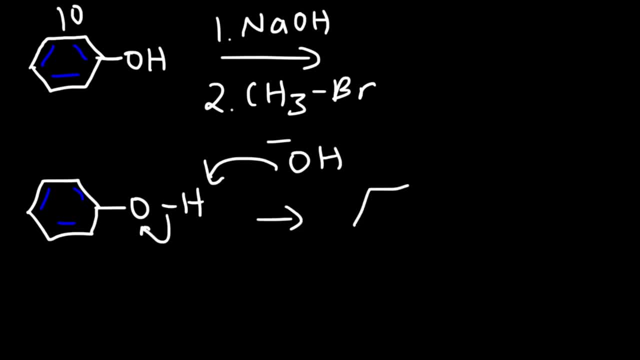 and the reason why phenol will take off the hydrogen is because the pKa for phenol is 10.. So in the first step, the pKa is more acidic than a typical alcohol is because the conjugate base is stabilized by resonance. The negative charge on the oxygen can delocalize into the ring, thus stabilizing 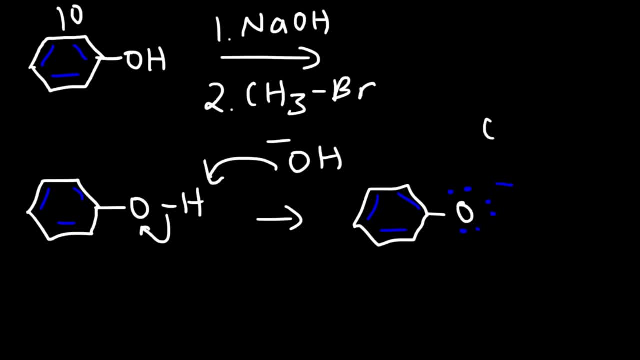 it In the next step. we can react phenoxide with methyl bromide, and so we're going to get an ether. We're going to get methyl phenol ether, And so that's another example of the Williamson ether synthesis reaction. Now let's go over another example. So consider this molecule. 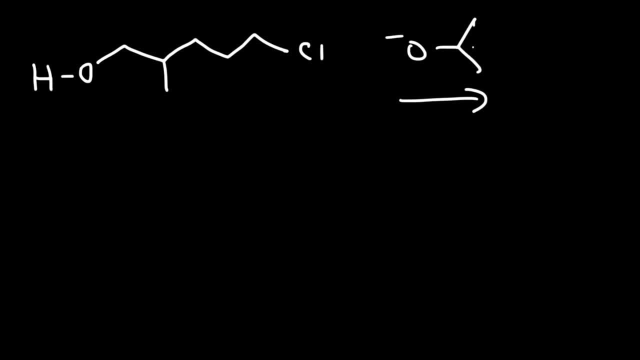 What's going to happen if we react it with tert butoxide? Go ahead and predict the major product of this reaction. There's two things that tert butoxide can do. It can behave as a nucleophile, attacking the carbon, kicking out the chlorine atom. Or it can behave as a base, abstracting the. 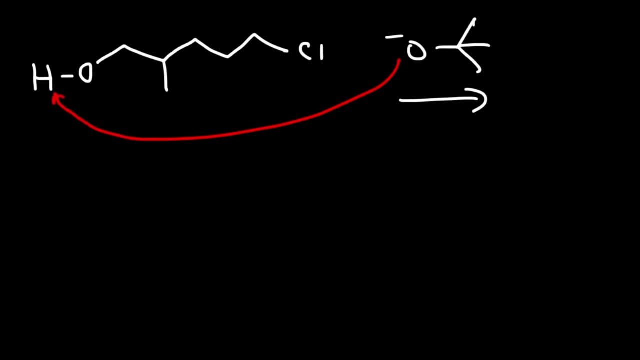 hydrogen atom And in fact, both of these things can happen. However, because tert butoxide is a bulky base, hysterically hindered due to all of these methyl groups, it prefers to behave as a base rather than a nucleophile. So by making the base more hysterically hindered, you can increase its specificity, You can. 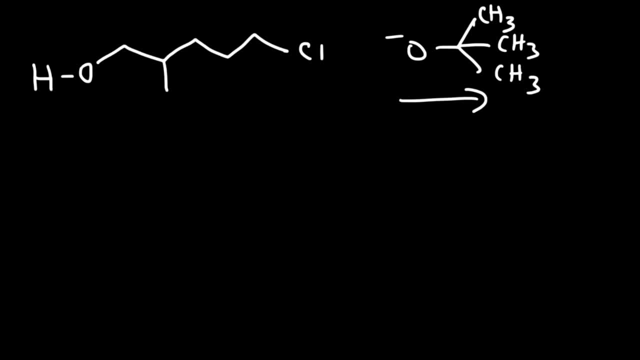 make it behave more as a base and less of a nucleophile. So we're going to focus on this reaction where it takes off the hydrogen. But just keep in mind that both things can happen, So you can get a mixture of products in this example. 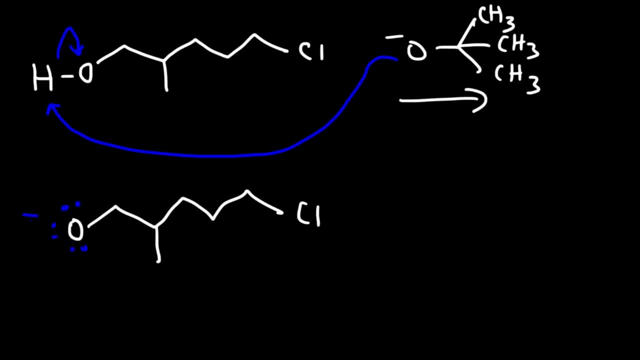 However, we can increase the yield of this reaction. this base more sterically hindered. there are other bases out there that is so sterically hindered that they don't act as nucleophiles, they just only act as bases. now, once we take off this hydrogen and we get the alkoxide ion, this oxygen, 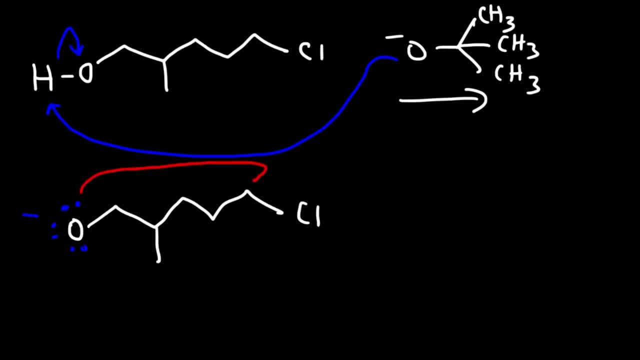 is going to attack itself- not itself, but it's gonna. the molecule attacks itself, and so you can have an intramolecular reaction and so it's going to close and form a ring. let's call this one, two, three, four, five, six. so we're gonna get a. 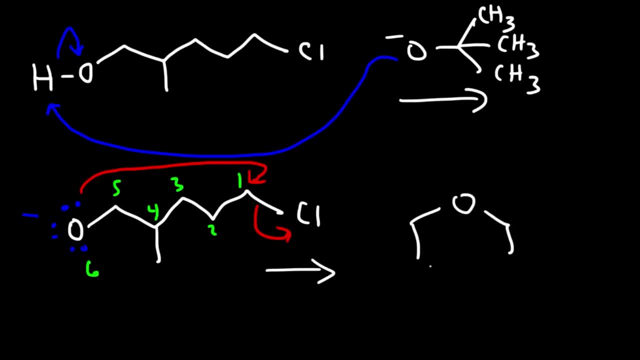 six membered ring. so let's say this is six. this is going to be one, two, three, four and five. attached to carbon-4. we're going to get a six membered ring. so we're going to get a six membered ring. we have a methyl group and this is basically it. so this is the final product. 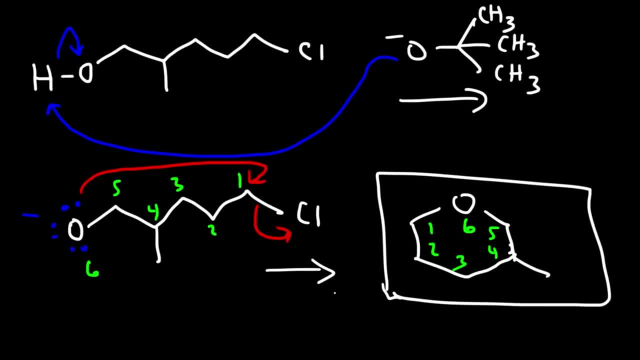 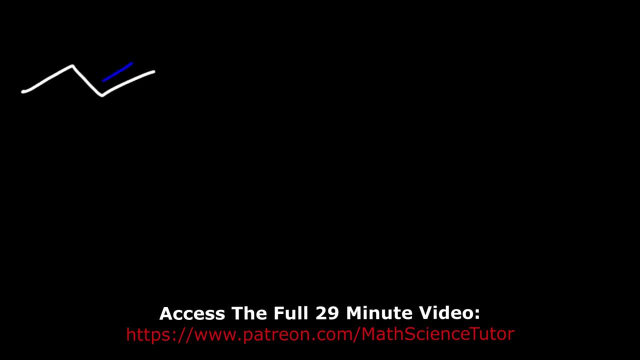 of this reaction. so we have basically an ether inside of a ring. now there are other ways in which we can make an ether, particularly if we start with an alkene. so if we react the alkene with methanol under acidic conditions, notice what can happen: the alkene will react with the hydrogen. 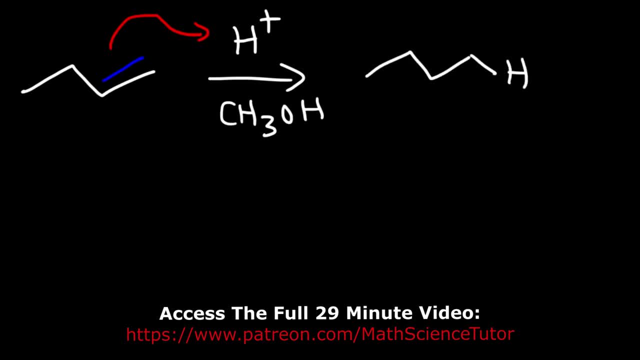 and the hydrogen will go on a primary carbon so that we can get a more stable secondary carbocation intermediate, and then the methyl molecule will attack the carbocation, and so we're going to get this species, and then, in the final step, another methanol molecule will take away this hydrogen, and so the end result is: 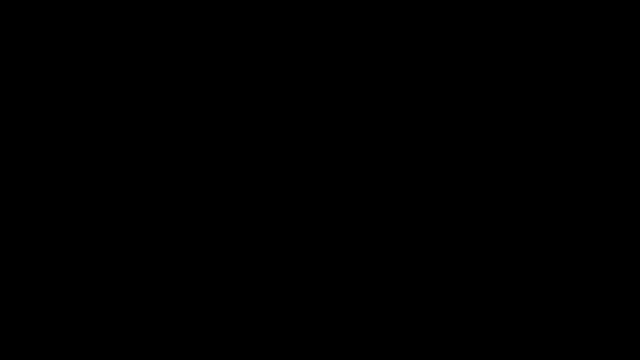 that we have an ether. another way in which we can make an ether is the oxymercuration demercuration, actually the alkoxymercuration demercuration reaction of alkenes. so we're going to use mercury acetate with- let's use- ethanol, ch3, ch2oh, followed by 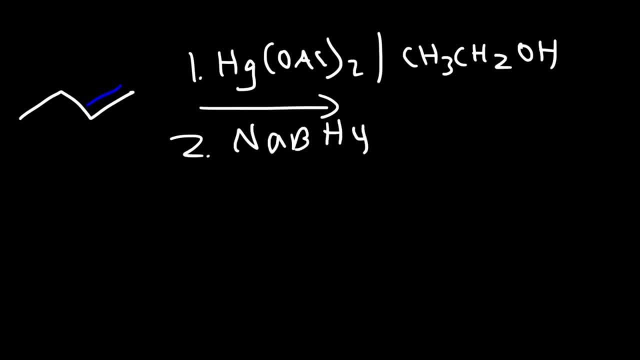 sodium borohydride. the end result is that we're going to add the ether here. on the secondary carbon. This reaction proceeds with Mccormick-Carvey geochemistry, And so all we need to do is take off the hydrogen and just add this group to the 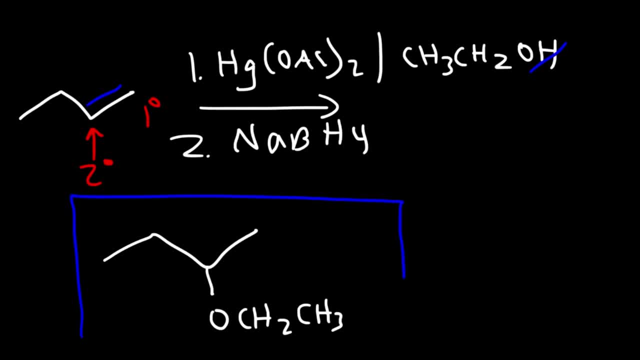 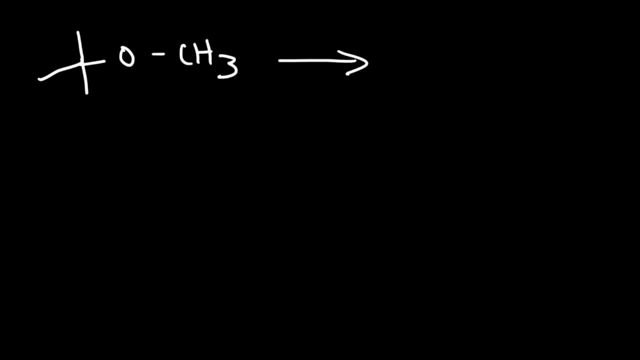 secondary carbon. So that's another way in which you can make ethers using the alkoxymercuration-demercuration reaction. Now let's talk about the acid catalyzed cleavage of ethers. Ethers don't react with bases for the most part. 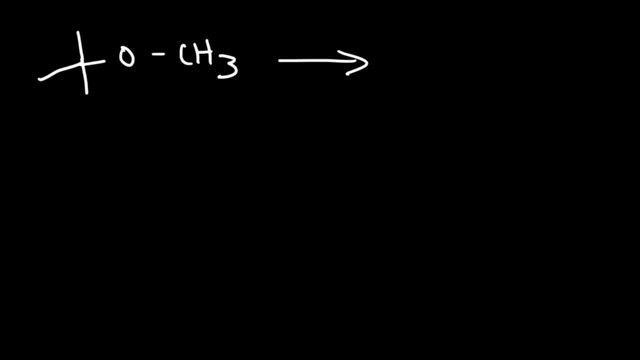 They're unreactive towards them, But to acids they tend to cleave. So let's react to this ether with hydroiodic acid. What do you think is going to happen? Now? you need to determine if the reaction will proceed by an SN1 mechanism or an. 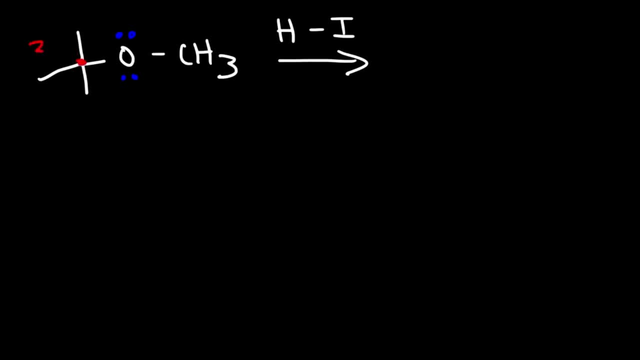 SN2 mechanism. So notice that this carbon is tertiary, which means that the reaction will proceed by an SN1 mechanism or an SN2 mechanism. So notice that this carbon is tertiary, which means that we can get a fairly stable tertiary carboketa intermediate. So 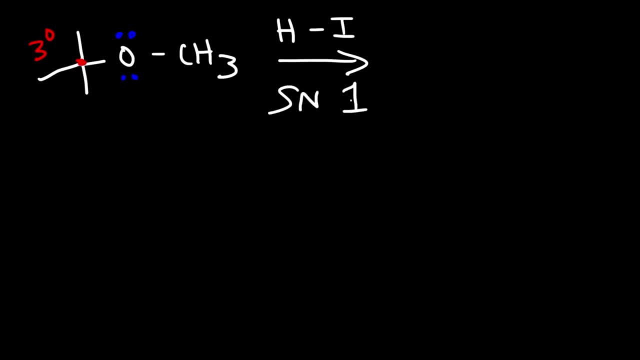 therefore, this reaction is going to go via the SN1 mechanism. The first step is protonation. The purpose of this is to make the oxygen a good leaving group, And then, in the next step, the oxygen is going to leave, And so we're going to get a tertiary. 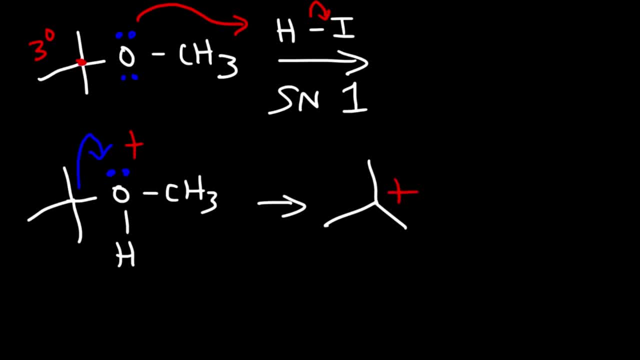 carbokedon intermediate, And the first side product that we have is methanol, And then, in the second step, iodide will come in, giving us an alkohalide, And so these are the two products that we get in this reaction If we add one equivalent. 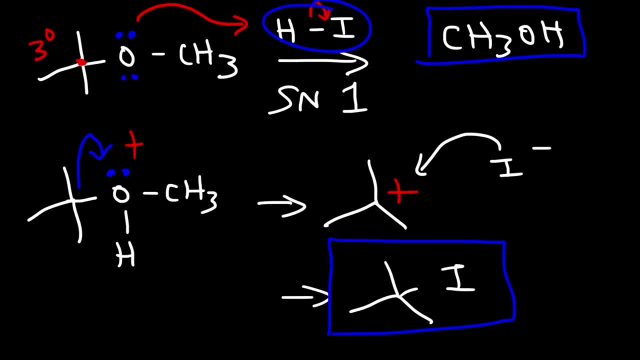 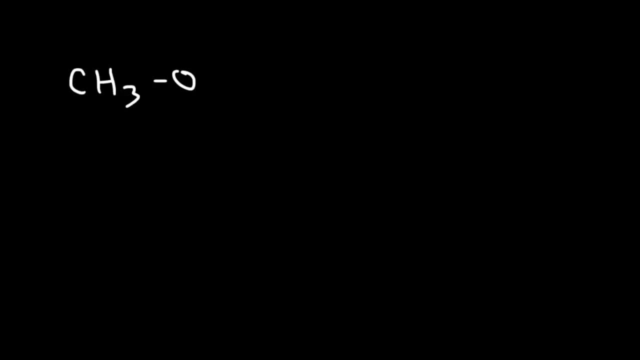 of HI. Now it's important to understand that if we add excess HI, it can react with methanol. So if we add another HI molecule, then this oxygen will be protonated in the first step. By the way, this will occur by an SN2 mechanism. 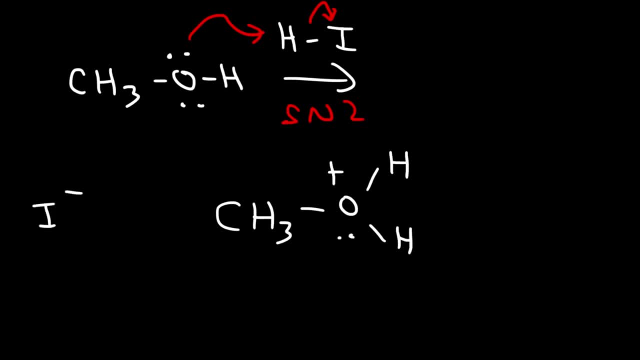 So we're going to get this intermediate and then, in the second step, iodide is going to attack from the back in an SN2 reaction, kicking out the water molecule given methyl iodide. So let's summarize what's going on here. 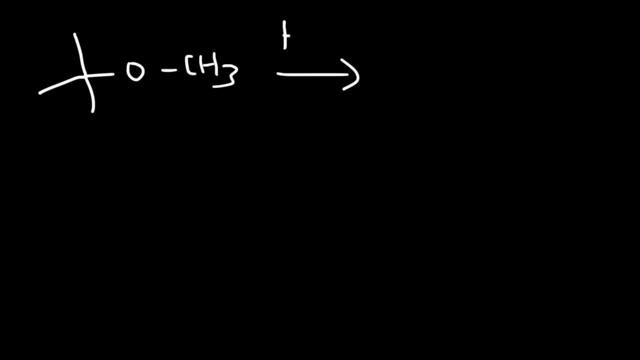 So let's say, if we add HI in a one-to-one reaction with this ether, or basically if we add one equivalent of it, then we're going to get these two products: Tert-butyl iodide and methanol. So the iodide ion will go on the tertiary carbon. 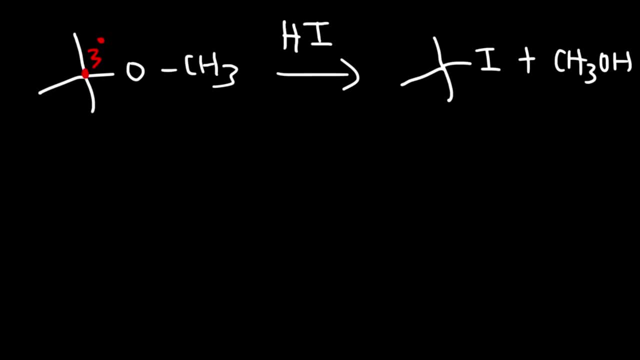 It's going to go on the more substituted carbon of the ether. Now if we add to the same ether excess HI, this reaction will go to completion. We're still going to get tert-butyl iodide, But it's going to react with methanol, giving us methyl iodide.